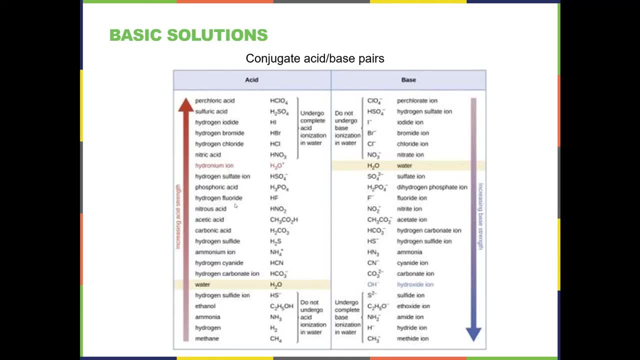 So Hf is a relatively weak base. So we have a conjugate acid-base pair here, where they're both relatively weak acids and bases. Then let's go to a more extreme case down here. Water is a very weak acid Hydroxide. its conjugate base- OH- is a strong base, as we just talked about before. 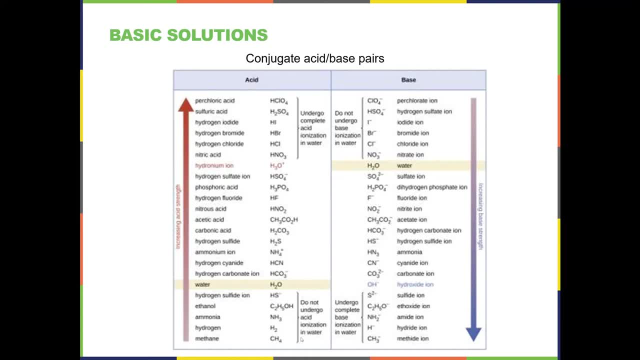 And then there are bases that are even stronger than HCl. So HCl- is a weak acid and HCl- is a strong base, as we just talked about before. And then there are bases that are even stronger than OH-. However, you're not going to find 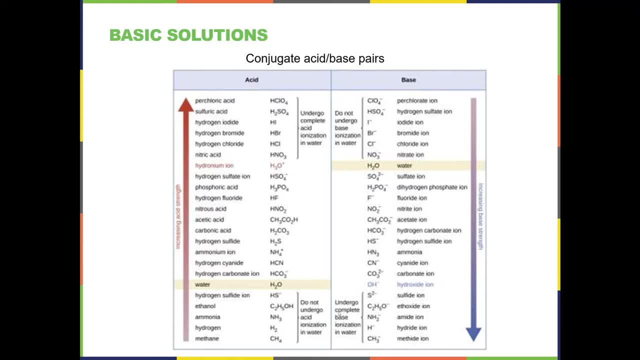 these things in water, okay. So basically what's going to happen is, if you mix these with water, they'll start stealing protons from the water. So in aqueous solution, we usually go in this range up here and we don't really consider these ones. So this is basically what we're looking at here. 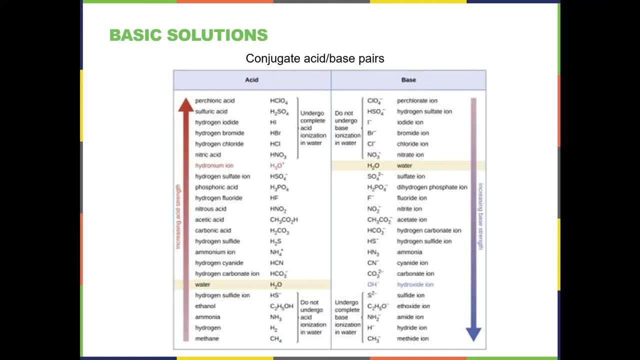 And what we want to talk about is how do we deal with bases, now that we've already dealt with acids, And there are several things to consider. Fortunately, these things are very similar to how we deal with acids. They're just a little bit different. So 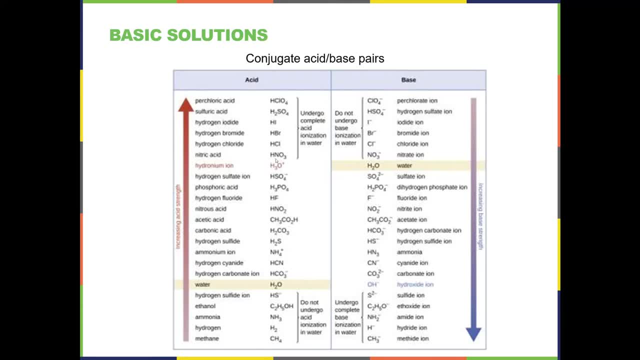 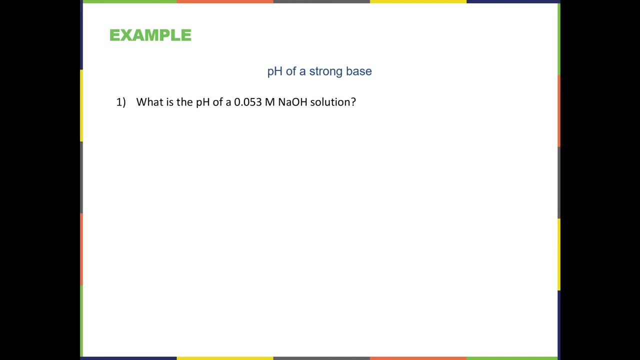 let's take a look. We'll both do some examples and talk about some theoretical kind of stuff. So the first one is: what is the pH of a 0.053 molar NaOH solution? And NaOH is one of those six strong bases that we talked about earlier. 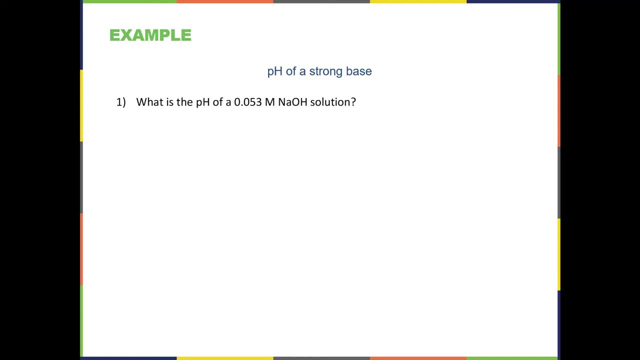 Because it directly puts hydroxide in solution. Said another way, if I have NaOH solid and I dissolve it in water, I get Na plus aqueous plus OH minus aqueous. Note that if this is 0.053 molar, 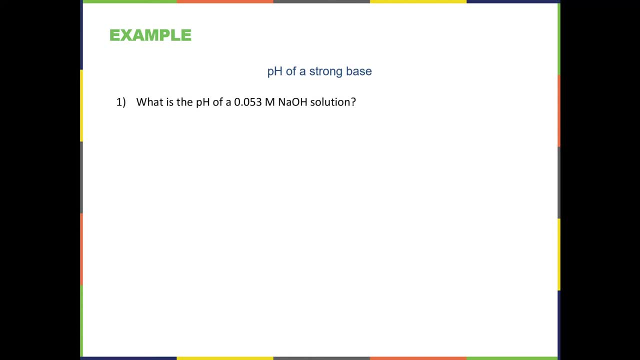 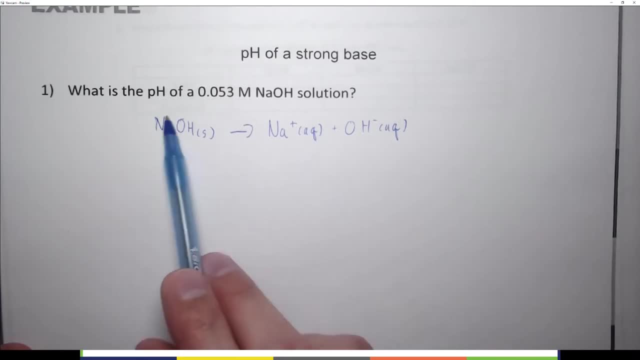 this is 0.053 molar Because, oh you know, it would help if I showed you what I was talking about. Note that if NaOH is 0.053 molar, OH minus is 0.053 molar. So these things have the same. 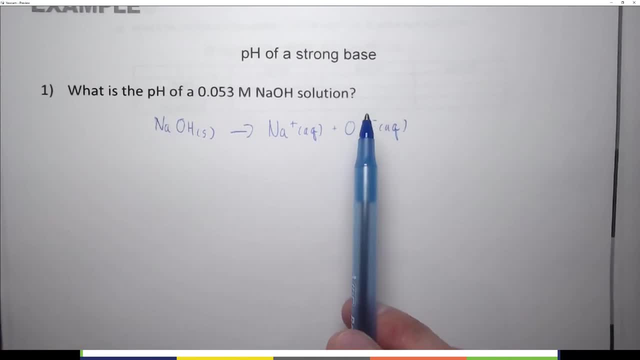 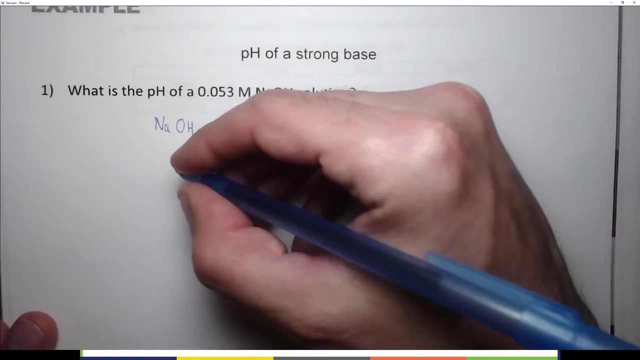 concentration in solution. Well, if I want to find the pH of this solution, I have two choices: I can find the concentration of H3O plus, or I can find the pOH and then find the pH. In my opinion, it's easier to find a pOH first and then convert it into a pH. 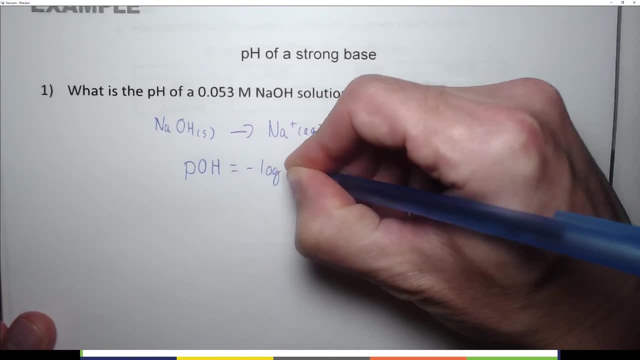 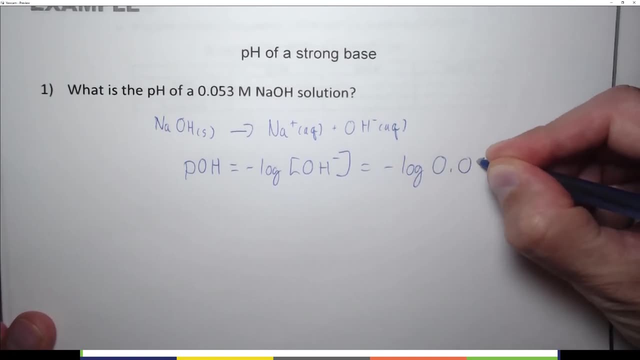 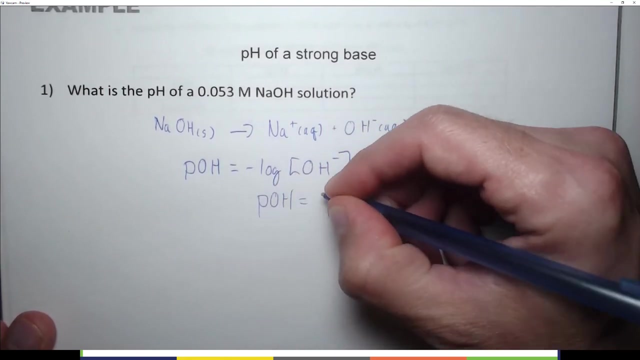 The pOH equals the negative log of the concentration of OH minus, which equals the negative log of 0.053 molar. And when I do that math I find that the pOH equals 1.27.. All right, so this is a strongly. 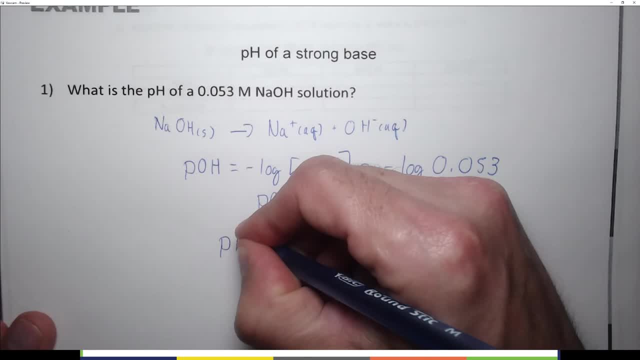 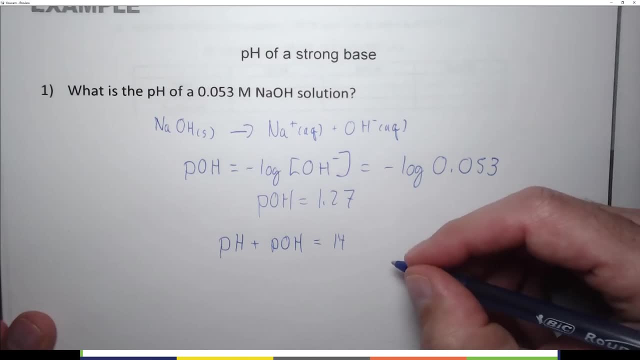 basic solution. Well, if you remember from the previous section a couple of seconds ago, pH plus pH equals 14, or said another way, pH equals 14 minus the pOH, And when I do that math I take 14. 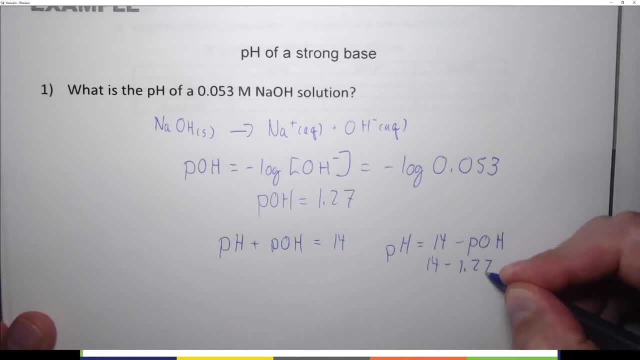 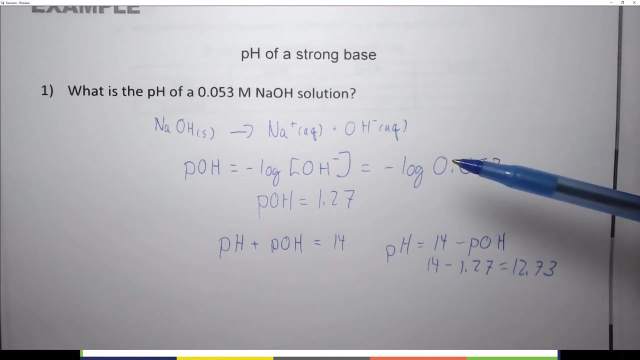 minus 1.27. And when I do that I get 12.73.. Very much like when we added HCl in a previous example, in a previous section of this chapter. we didn't use a Ka expression. We didn't use a Ka expression to figure out the pH of an HCl solution, because HCl is a strong acid. 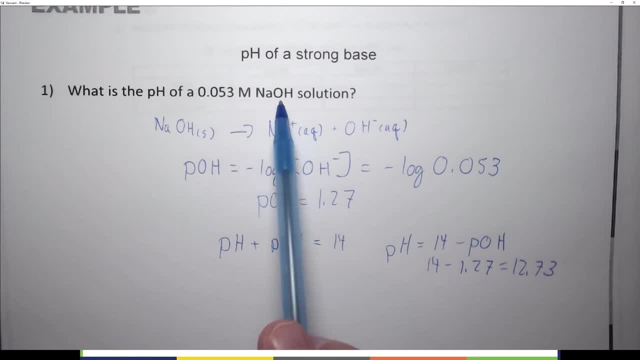 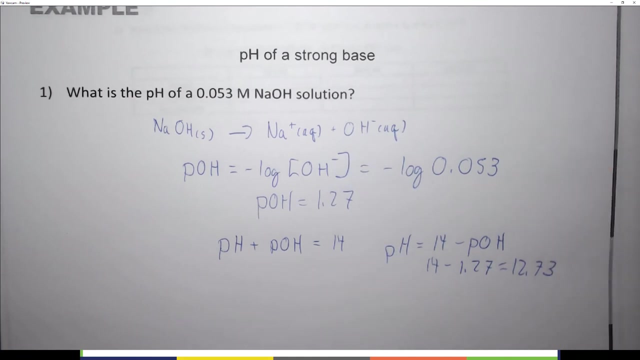 Same for strong bases. We don't use a Kb expression in order to find the pH of the solution, because these are strong bases. They're not interacting with water weakly. Whatever the concentration of this is, that's the concentration of this and we can find the pH directly from that. 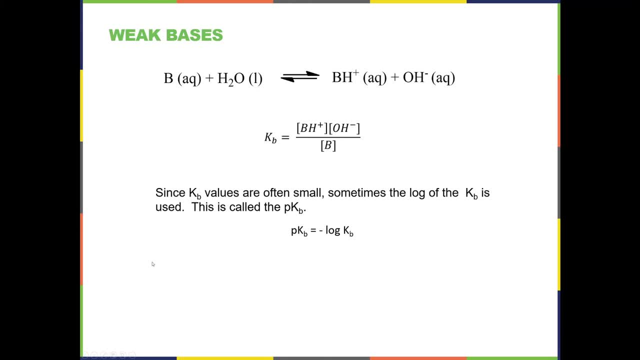 value. So next we want to look at what do we do with these weak bases, And we'll go through a few examples of those as well. Well, in this case we have B interacting with water and B is aqueous. 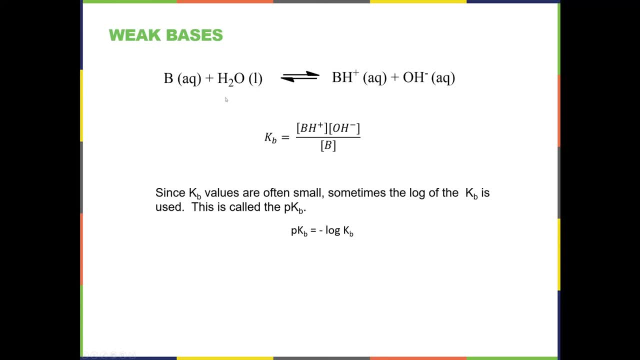 and it forms BH plus. So this acts as a base, taking a proton away from water to form BH plus. So we have B plus an H and a plus charge. So we gain an H and a plus And what's left? Well, 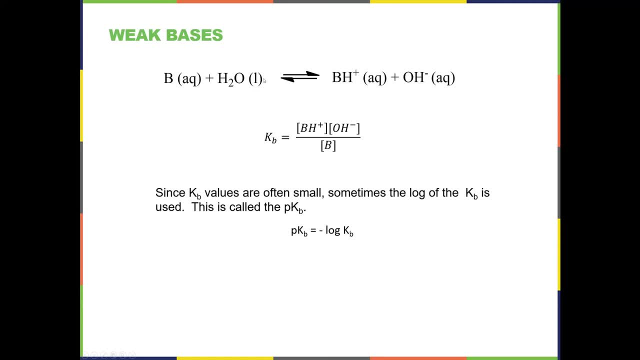 we lost an H plus, So we have one less: HOH instead of H2O, So this has two H's and this only has one. We lost that H and we gained the minus charge because the H plus left- It left its electron there, So this has a minus charge. 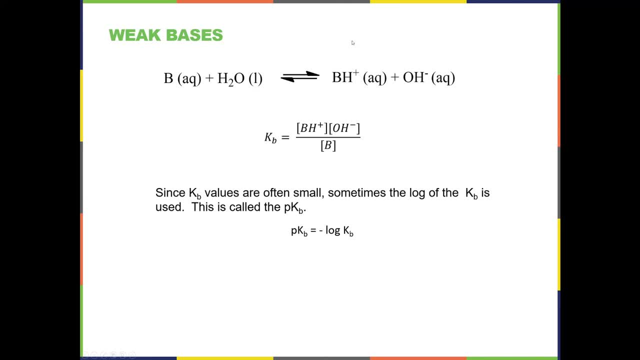 Another way of looking at this is: overall it's neutral here. Here we have a plus and a minus. Overall, it's neutral here. Well, we can write the Kb expression for this, just like we wrote the Ka expression, And I don't think it's a big surprise that it's still products over reactants. So in 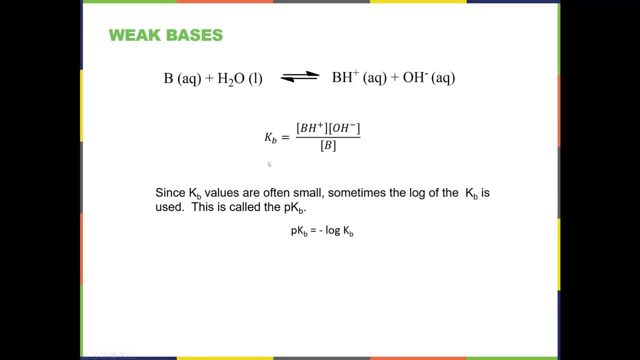 this case it's BH plus over OH minus all over B. Okay, B does not have to be neutral. Okay, sometimes it does, And you'll have B minus plus H2O and you'll get BH with no charge plus OH minus. So 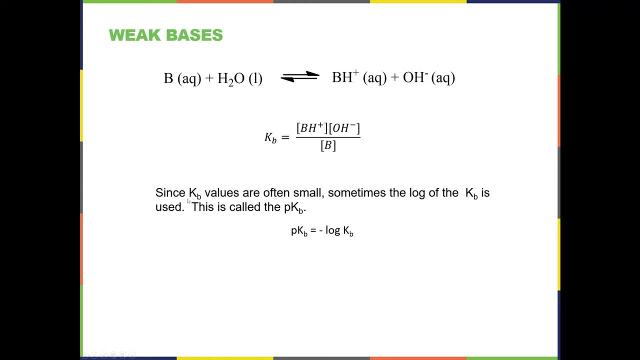 that's also a possibility. Since we have the Kb here, we can take the negative log of it and get the PKb. just like we did for the Ka, We could get the PA- excuse me, the PKA. So this is basically. 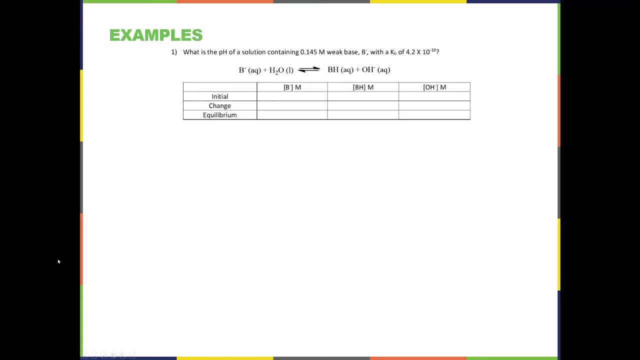 how that works. Now let's look at an example, And this time I'm going to remember to switch over to the camera. So let's look at an example, And this time I'm going to remember to switch over to the camera. And this time I'm going to remember to switch over to the camera, And this time I'm going. 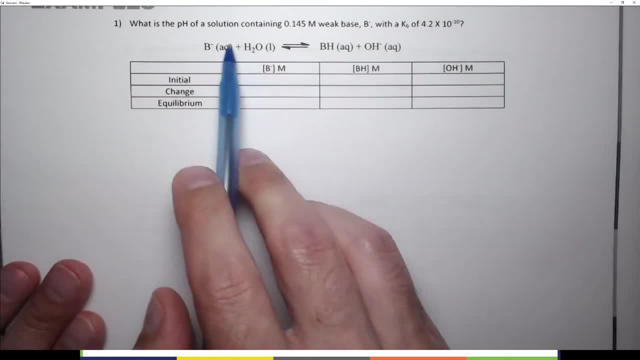 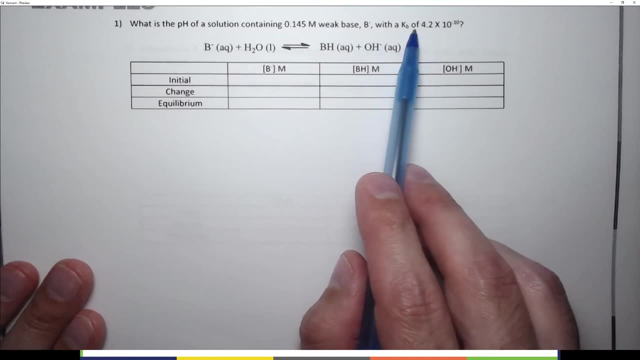 to remember to switch over to the camera So you can actually see what I'm writing. It says: what is the pH of a solution containing 0.0145 molar weak base B minus with a Kb of 4.2 times 10? 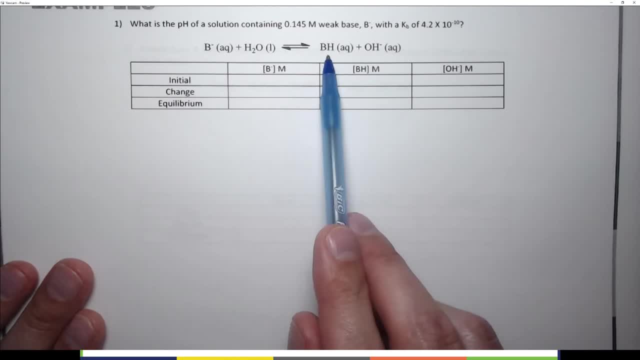 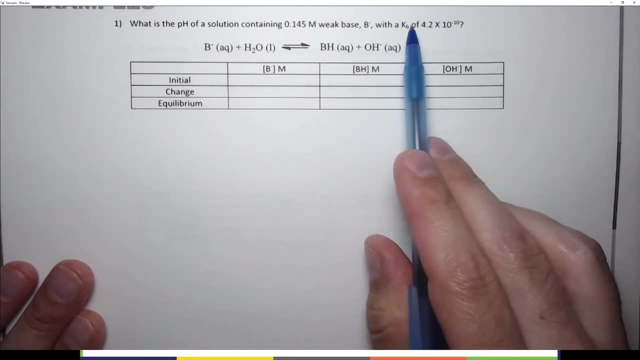 to the minus 10.. And now we have B minus plus H2O yields, BH plus OH minus. Now this is very similar to a Ka problem, It's. the only difference is we're using a Kb, And you're going to see at the end. 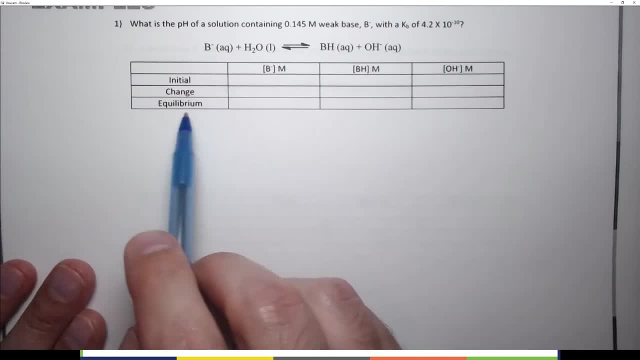 there's a little bit of a difference in calculating the pH. We have another ice table. We've used these lots of times So I'm not going to spend a whole lot of time on it, But I do want to fill it out. We have everything that's aqueous in our ice table. We 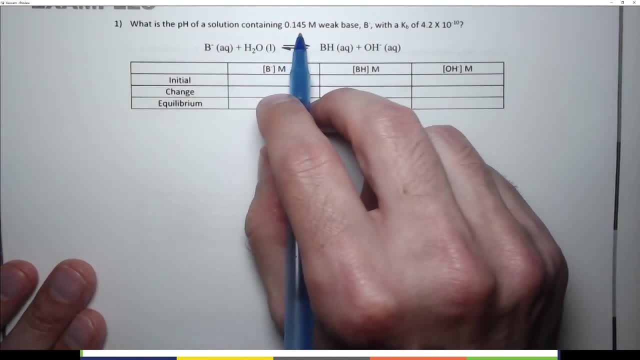 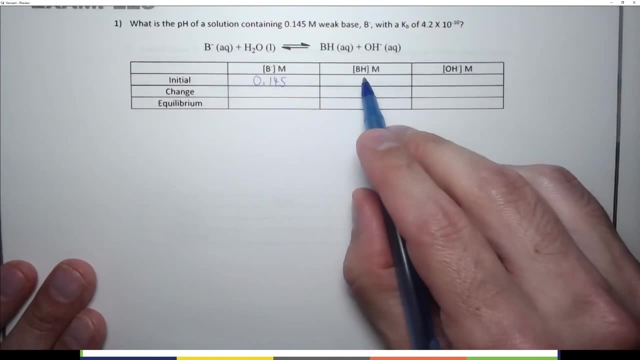 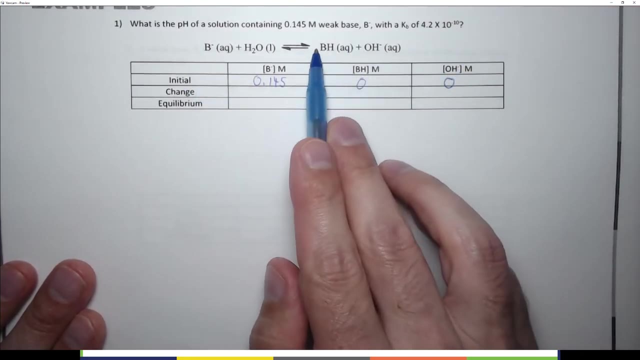 don't have water. as usual, We know the original concentration of B minus because it tells us so it's a 0.145 molar. As usual, the initial concentration of BH and OH minus are zero. So we start the reaction with only B minus And then, as the reaction proceeds, we get some of 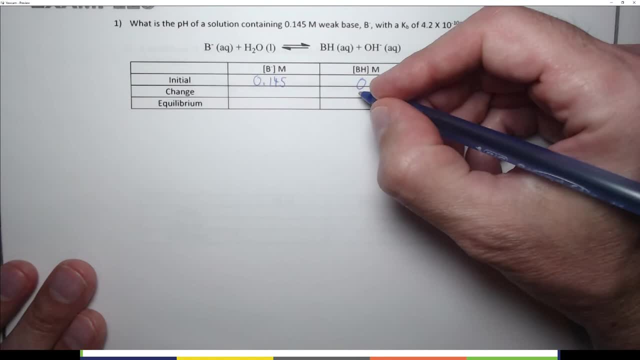 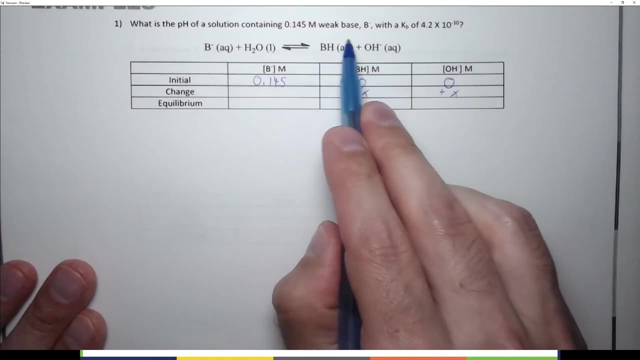 these two things We're going to change. Well, we don't know how much we're going to gain, So we'll call it X If we get X of this. as usual, we also get X of this, because it's a one to one stoichiometry. 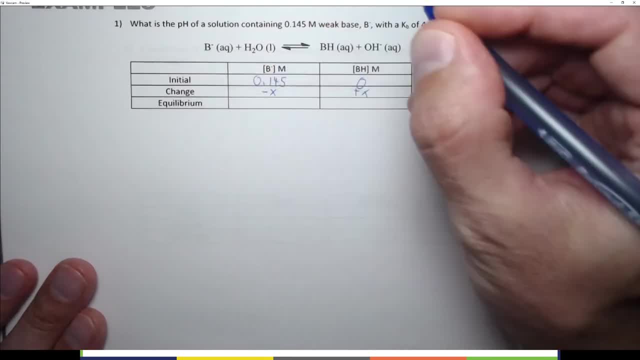 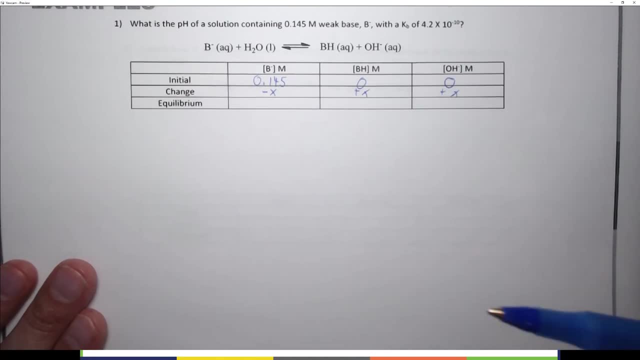 In this case the B minus. we're going to lose X of it again because it's one to one stoichiometry, just like the percent ionization problem in the previous section or in several of the examples in two previous sections. All right, 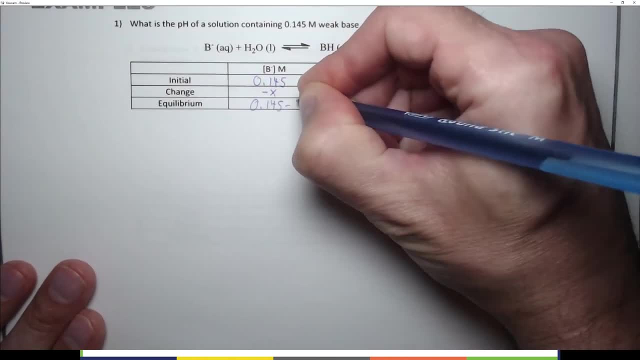 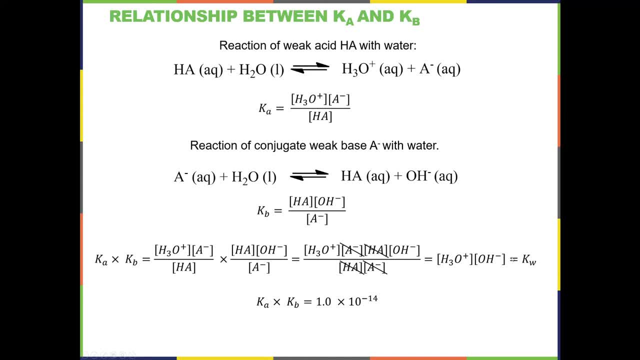 Remember that, generally speaking this: if this is less than 5% of this, you're allowed to ignore X. Remember that, generally speaking this: if this is less than 5% of this, you're allowed to ignore X. khK, b is k, ¿, ו'' and the value of their W is 1-10. 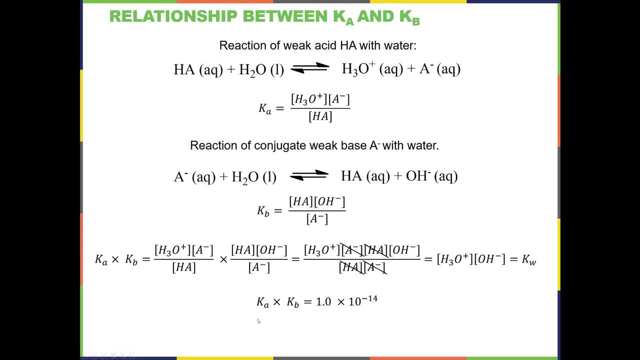 khK b is k Wh of its conjugate base. If you know the kh Weak base, then you can find the kh Acid, so you can convert from one to another through a constant as derived from the formula here. That's useful. Before we talk about that, though, there's a little bit of strangeness that. 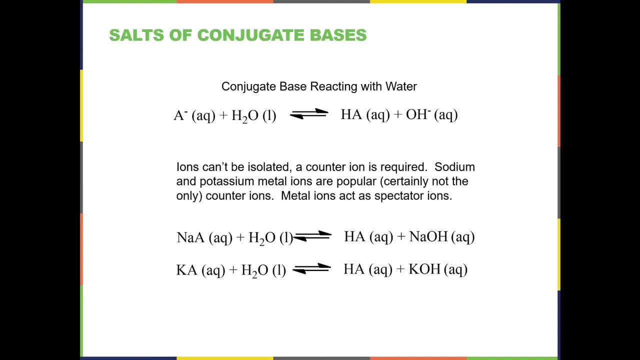 sometimes causes confusion. It's not really strange, It just can cause confusion. I've noticed over the years, So I want to talk a little bit about it before we move on. Here's the reaction: exactly the same that I had before. We have the conjugate base A minus. 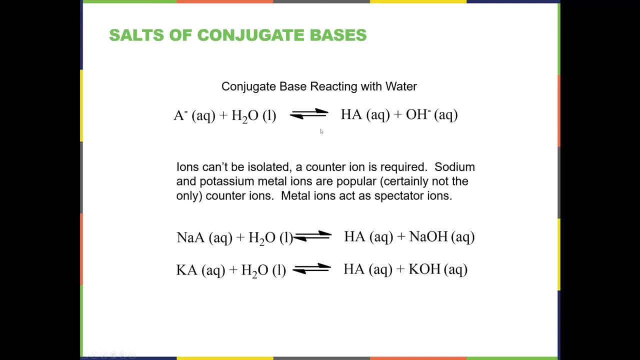 reacting with water to form HA and OH minus, just as I talked about before. But let's say I want to put some A minus into water. Turns out you're not going to be able to do that. okay, And the reason you're not going to be able to do that is you can't buy a bottle of negative ions. That's impossible. 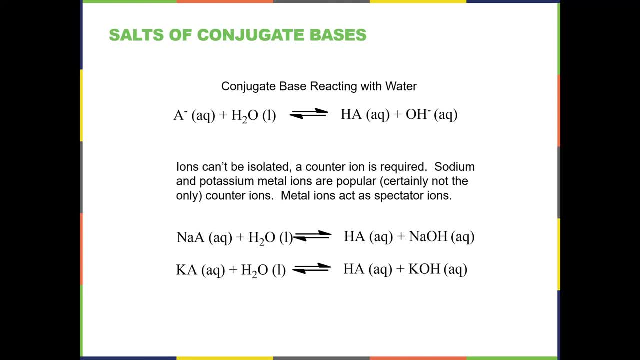 Remember, all ionic compounds are neutral when they're stabilized and you put them in a bottle. So if this was F minus, you can't buy a bottle of F minus and then put it in water. And when I say you can't buy a bottle of it, what I mean is it's not stable enough that one could put it in a bottle. 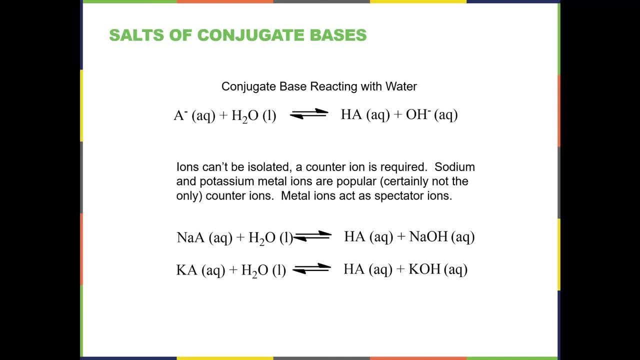 and you know then use it for whatever they wanted to use it for. The reason for that is: you can't have a bunch of negative ions next to each other. Well, how do you solve that problem? How you solve that problem is you need a bunch of positive ions to balance those out. 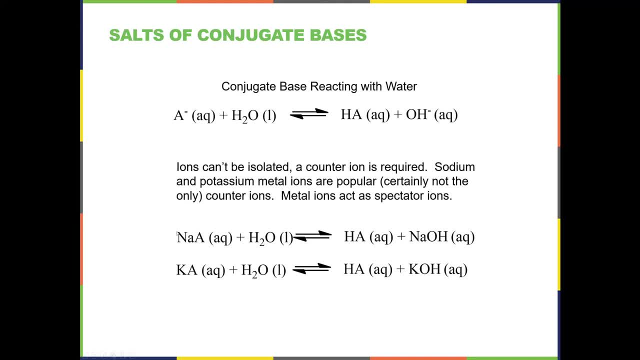 So if you have a minus charge, you need a positive charge to balance it out. You can't buy F minus, but you can certainly get a bottle of NAF alright, or a bottle of KF. So ions can't be isolated and put into a bottle. 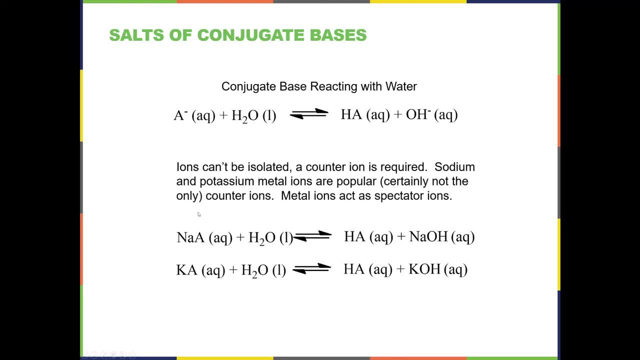 You always have to have a counter ion. So if you see NAA, what that really is is A minus, because when this dissolves, it breaks up into NA plus and A minus, as we've talked about in previous chapters. So 1A metals, sodium and potassium are not the only counter ions, but they're cheap and they work, and that's what we're going to talk about here. 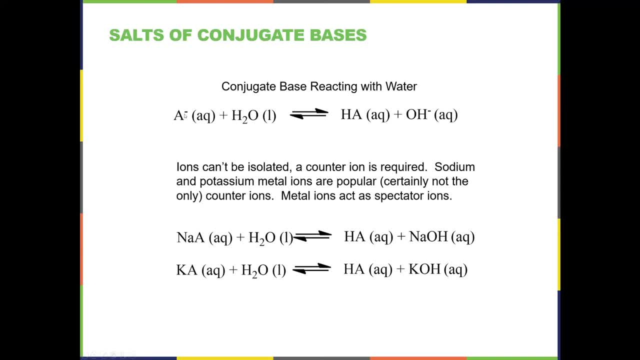 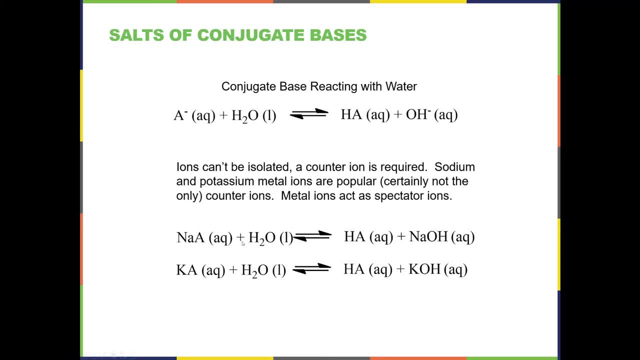 But sodium and potassium are the most common ones that we use. But sodium is pretty cheap, so maybe it's the most common ever. But sodium is pretty cheap, so maybe it's the most common ever. Alright, so let's look at an example. 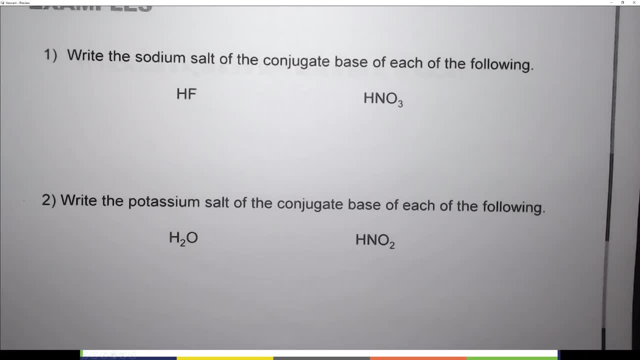 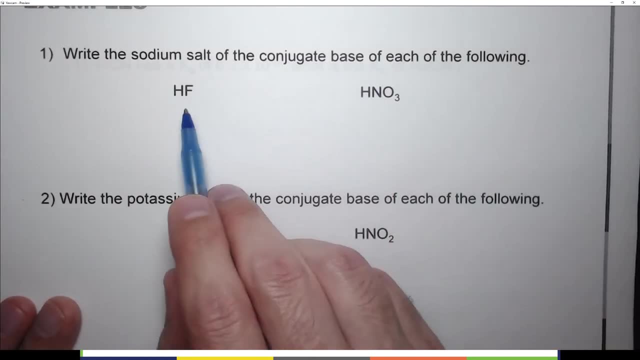 And I'm going to remember again to switch over to the camera here because I forgot a minute ago- It says: write the sodium salt of the conjugate base of each of the following. So, first step, what is the conjugate base of HF? 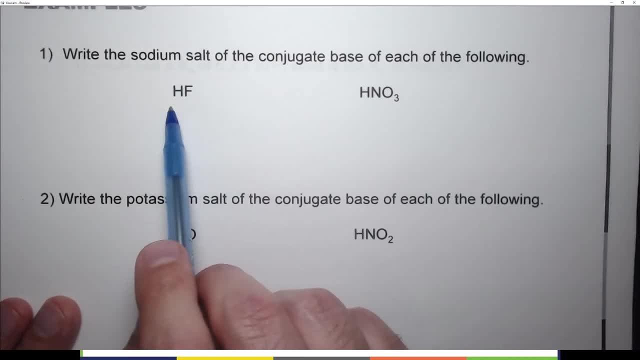 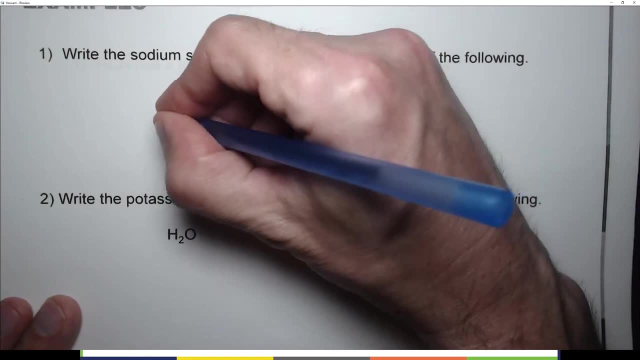 Well, if you want the conjugate base, HF has to act like an acid. What do acids act like? Well, if you want the conjugate base, HF has to act like an acid. What do acids act like? they're proton donors. So this has to lose an H and a positive charge. What's left? F minus Well. 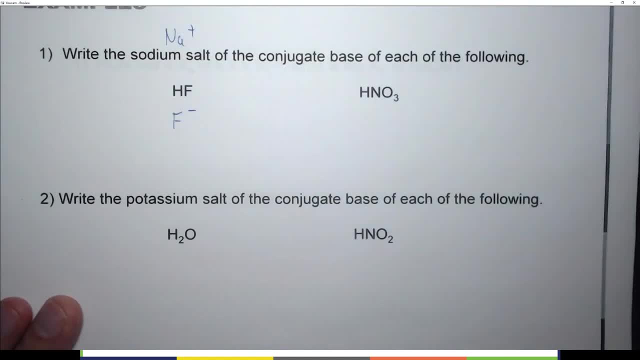 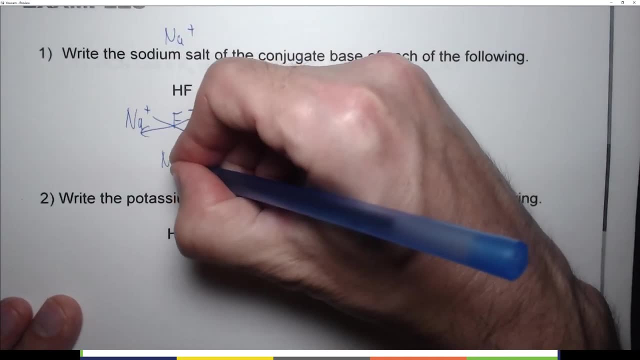 we want the sodium salt and sodium is a 1A metal, so it's Na plus. So we have Na plus, F minus. We cross the charges just like in Gen Chem 1 and we get NaF. So if you wanted to add to solution F, 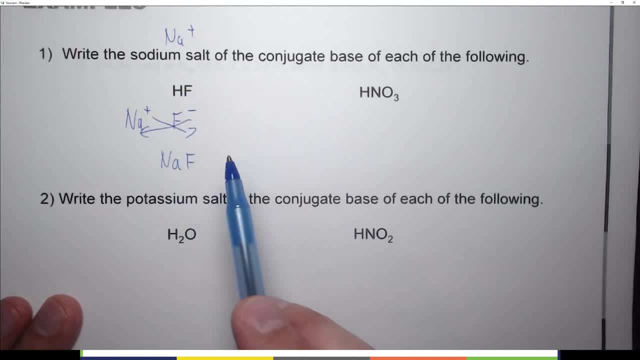 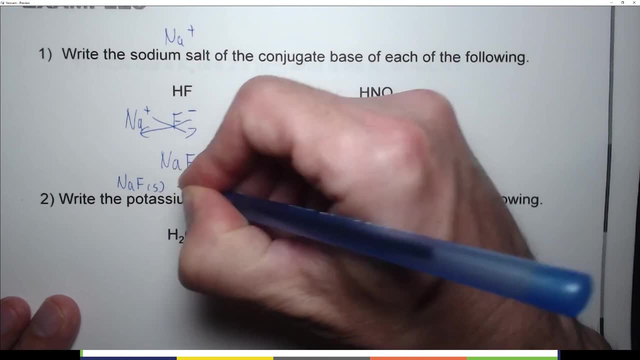 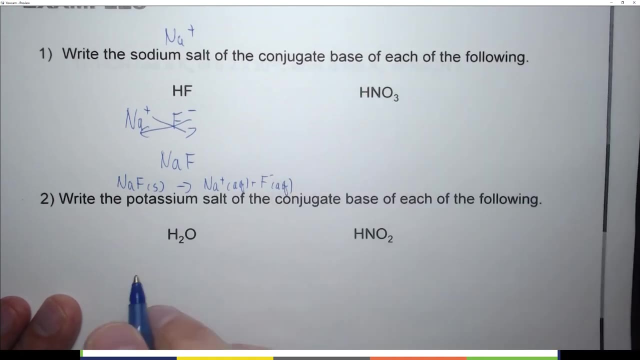 minus. you can't just get F minus, but you can get NaF and you can just add this and this will dissociate. It doesn't ask us for this, but NaF solid will dissociate into solution, into Na plus aqueous plus F minus aqueous. If you add a mole of this to solution, you will have a mole of F. 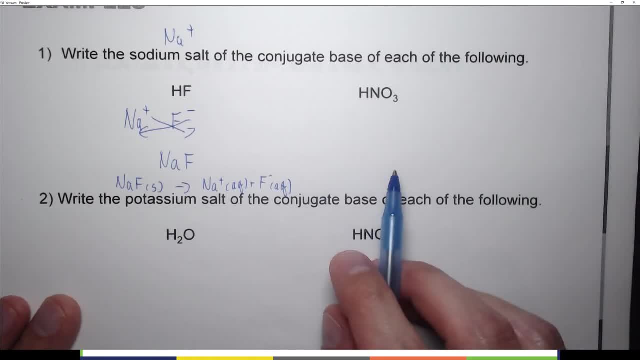 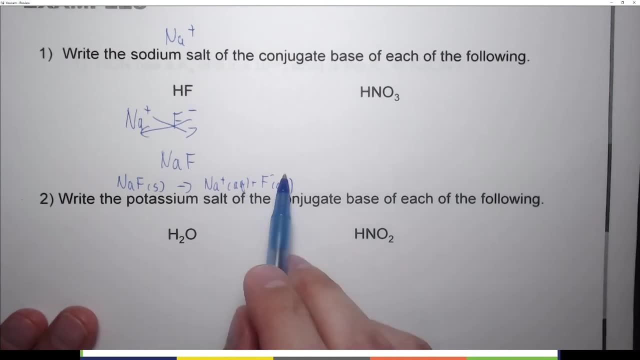 minus in solution and this works well, All right. this is another advantage of the 1A metals. 1A metals are always soluble, so that's helpful, because you need it to be soluble in order to get F minus in solution. If this doesn't dissolve, this does, but if it didn't dissolve, 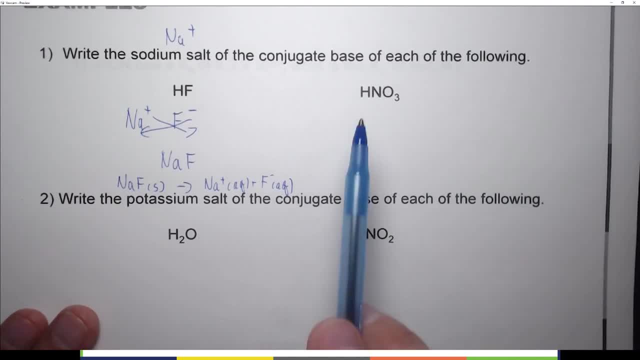 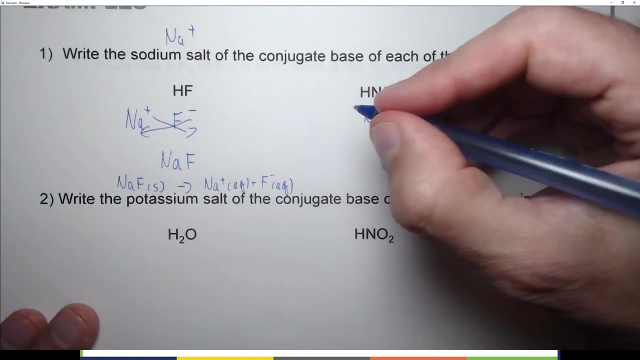 that wouldn't be very helpful. Let's look at HNO3.. What's the conjugate base of HNO3?? Well, again, to find the conjugate base, this has to act like an acid, and acids lose protons, so we get NO3 minus. What are we gonna have it with? Well, we're gonna have it with Na plus We cross them. 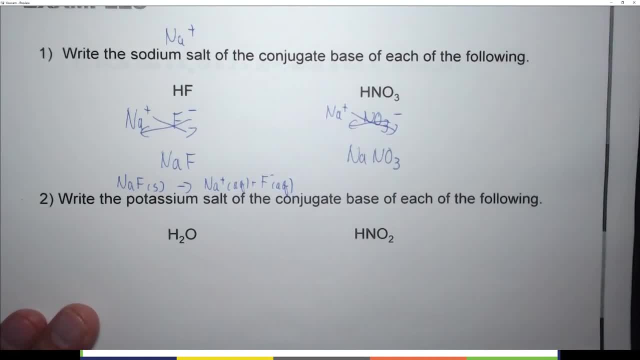 and we get sodium nitrate, NaNO3, which again breaks up in the same way as discussed before. Write the potassium salt of the conjugate base of each of the following. H2O has to act like an acid. What's left? OH minus. We don't usually write it as HO minus. We write it as OH minus. 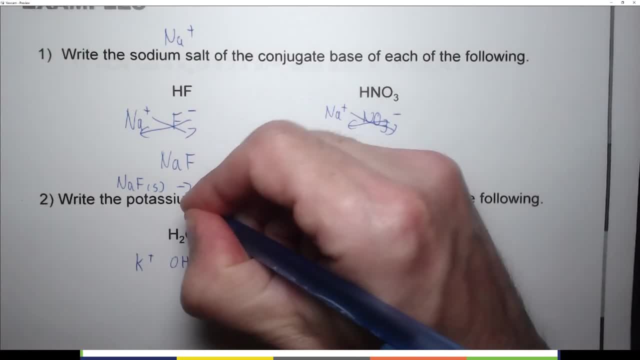 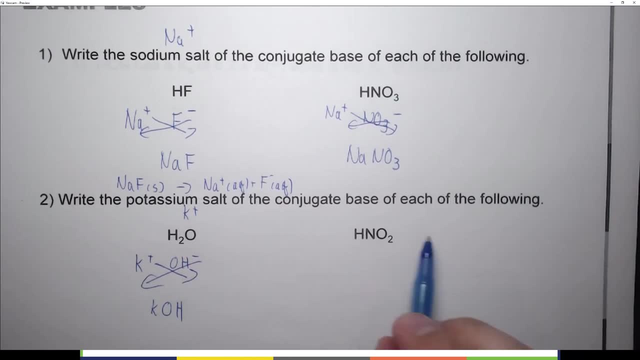 We have K plus. as the counter ion, Potassium, is just below sodium. It's a 1A metal, so it has a charge. We cross them and we get KOH. Finally, HNO2, nitrous acid, In this case the conjugate. 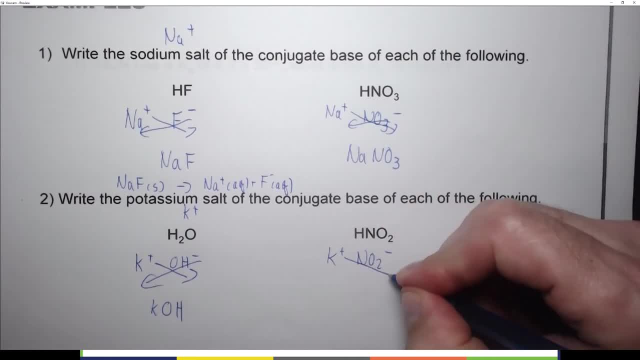 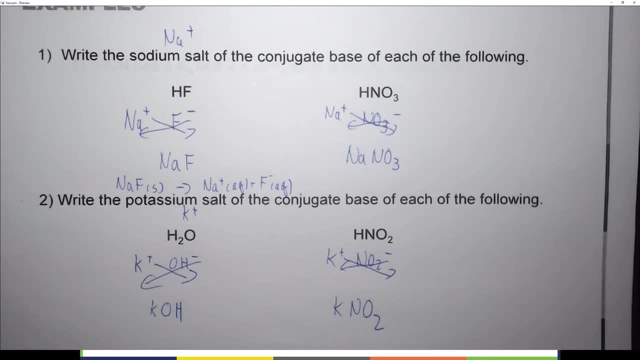 base is NO2 minus. We have it with K, K plus, We cross them and we get KNO2.. So if you see something asking you for the KB of F minus and it gives you the concentration of NAF, that is, the concentration of F minus, All right, so that. 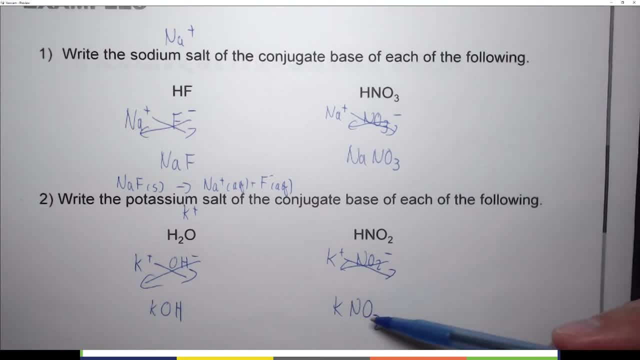 or, if it's, if it asks you about NO2 minus and it gives you KNO2. whatever the concentration of KNO2 is is the concentration of NO2 minus. You need a conjugate or a counter ion to balance out the charges and make something stable enough. 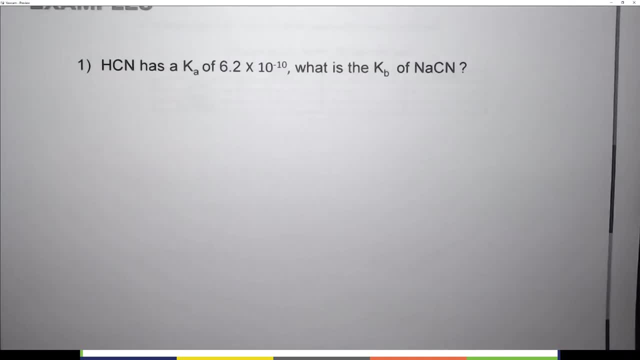 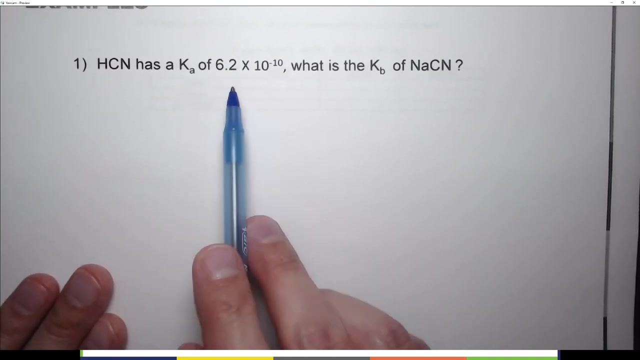 to put in a bottle. Here we have an example of. sorry, I don't know why I switched back over there. Here we have an example of this exact phenomenon. It says: HDN has a KA of 6.2 times 10 to the minus 10.. What is the? 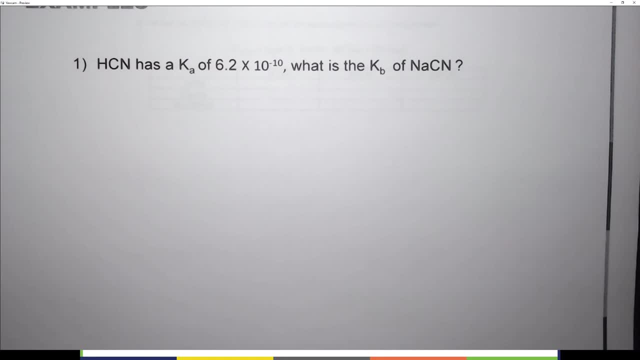 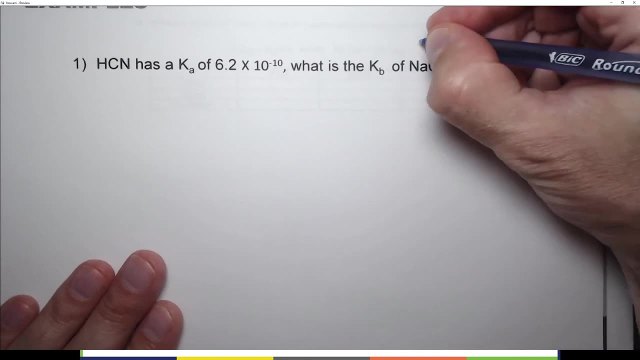 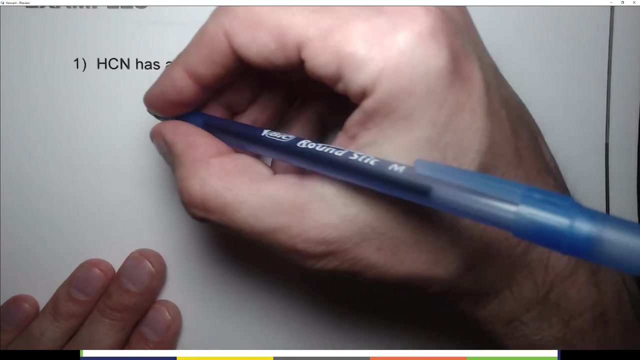 KB of NA. So, as we just discussed before, NA has nothing to do with this. NA is just a counter ion. It's going to be a spectator ion, if you will. What we really want is the KB of CN minus, If you remember before. 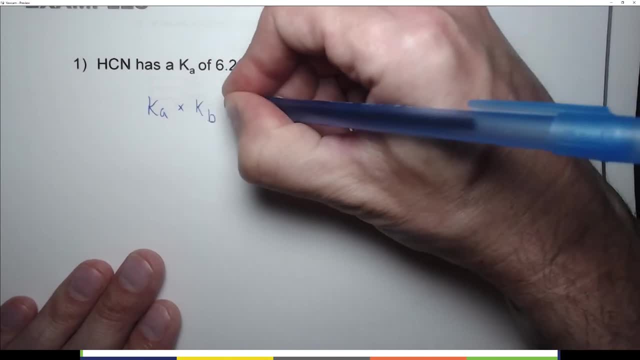 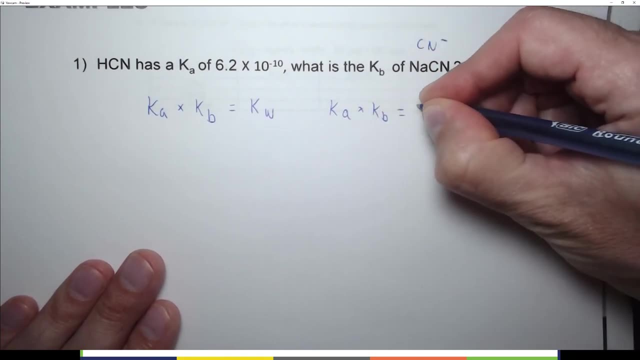 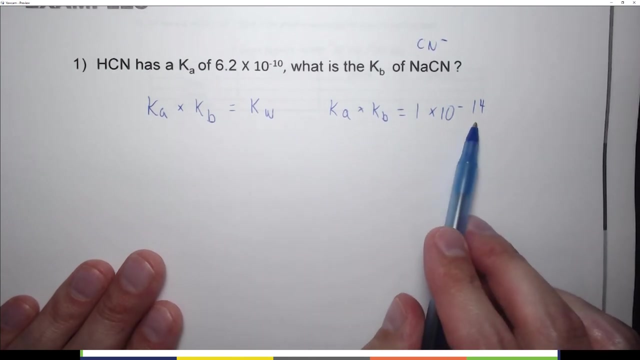 KA times KB equals KW, or KA times KB equals 1 times 10 to the minus 14.. All right, KW is a constant which has a value of 1 times 10 to the minus 14.. So, in order to solve this, we need: 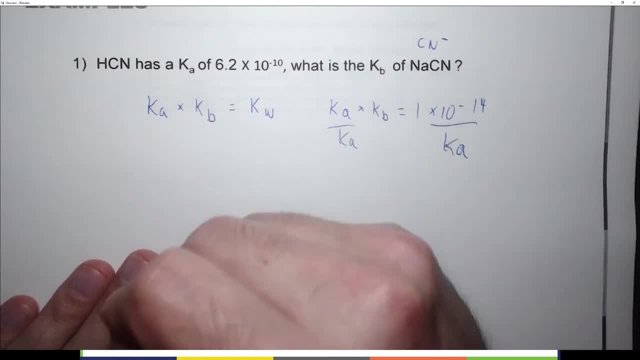 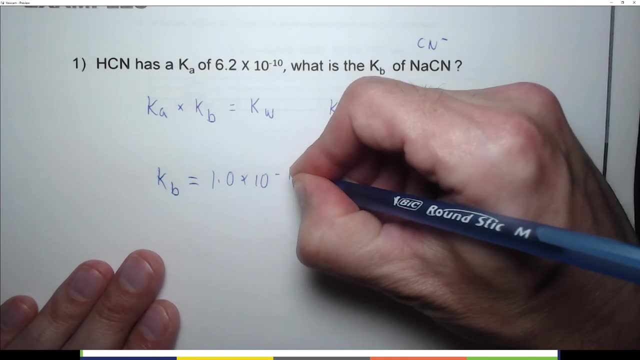 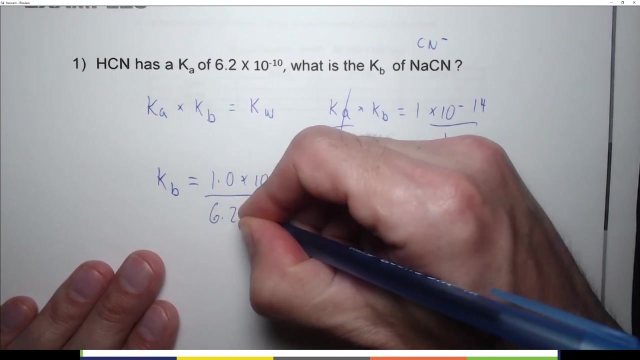 to divide by KA. divide by KA and we find that KB is equal to 1 times 10 to the minus 14. divided by the KA, that cancels out there, which is 6.2 times 10 to the minus 10.. And when we do that math we 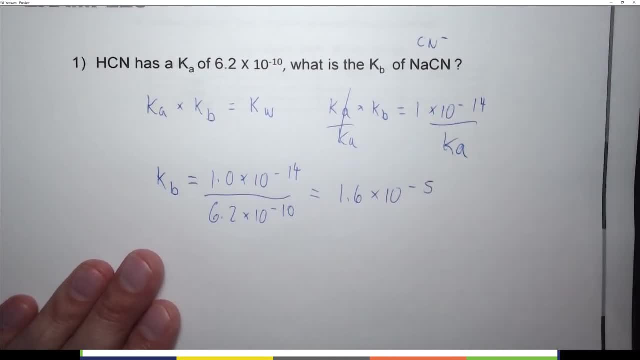 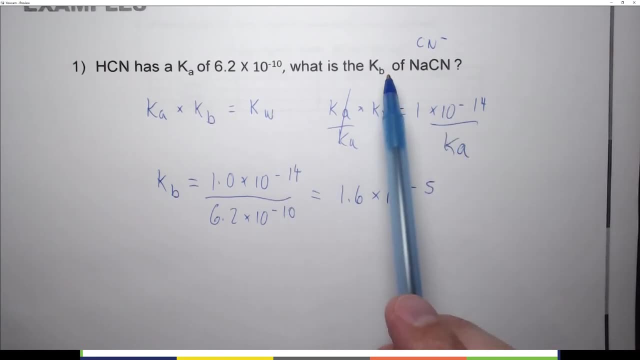 find that is 1.2 times 10 to the minus 10.. So we have a constant of 1 times 10 to the minus 14.. 0.6 times 10 to the minus 5.. If you notice, because of this mathematical relationship between KA and 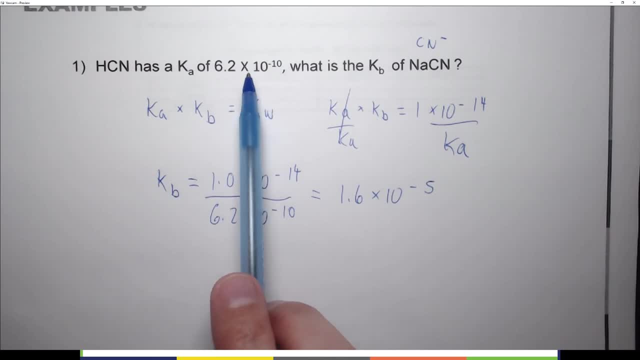 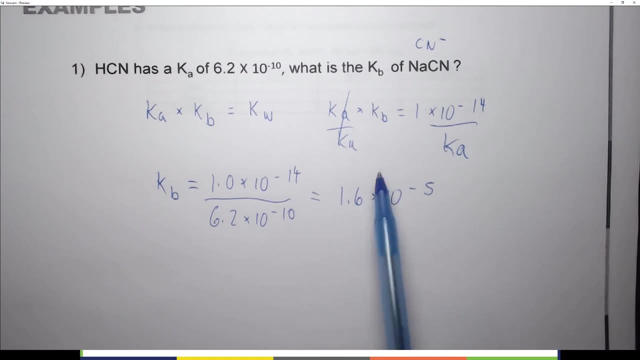 KB. the smaller that this value is okay, the bigger this value will be. Said another way: the acid and strength are reciprocals of each other, Meaning that if HCN is a strong acid, CN minus will be a very weak base. If CN minus is a strong base, HCN will be an even weaker acid. 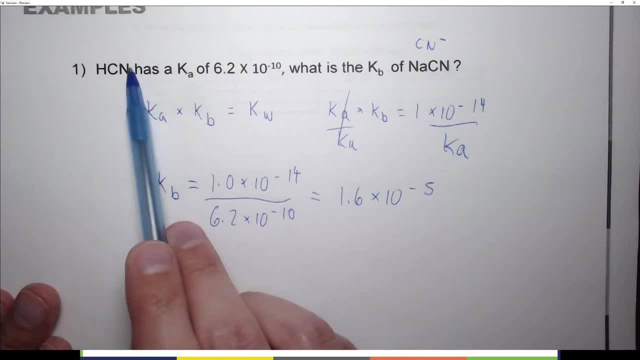 Why is that? Because they're doing the opposite of each other. If HCN really wants to get rid of a proton and is a stronger acid, then CN minus, which is trying to gain a proton, is going to be a very weak base and not very be very good at that, and vice versa If CN minus is a strong base. 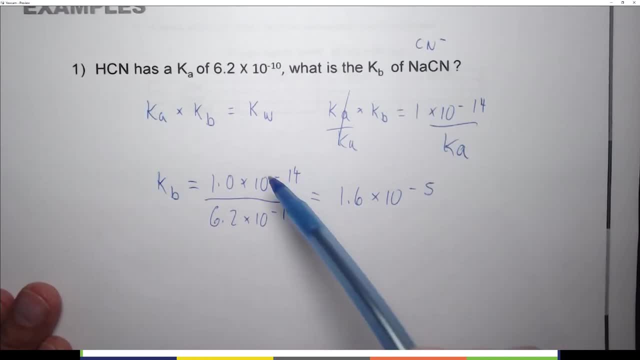 to gain a proton, then HCN is not going to be a very strong acid. So because of this mathematical relationship, we're going to have a very strong base and a very weak base. So we're going to have a. you can see, this KA is pretty small. this KB would be higher up on the scale, So CN minus would be. 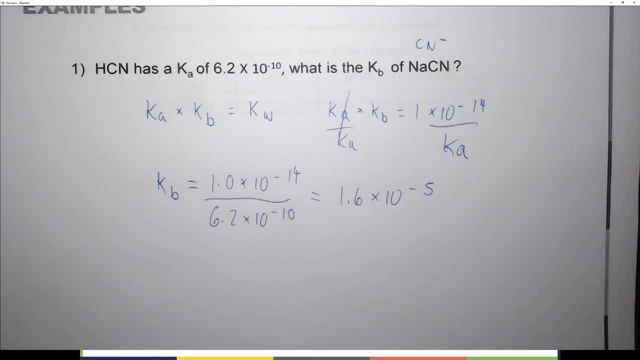 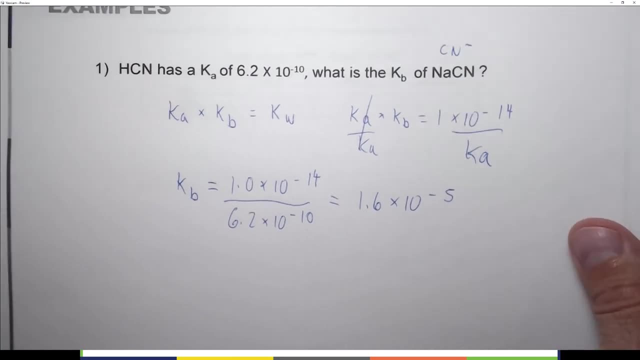 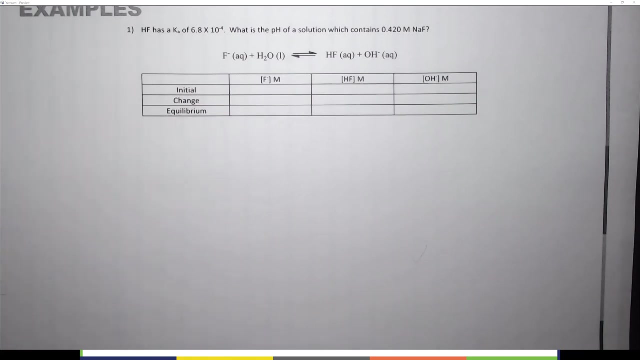 kind of strong, weak base, if you will. All right, which I understand doesn't quite make any sense, but this is the general idea in those trends that we talked about before, Finally putting it all together and doing a base problem which has both steps: using an ice table and converting from KA to KB. HF has a KA of 6.8 times. 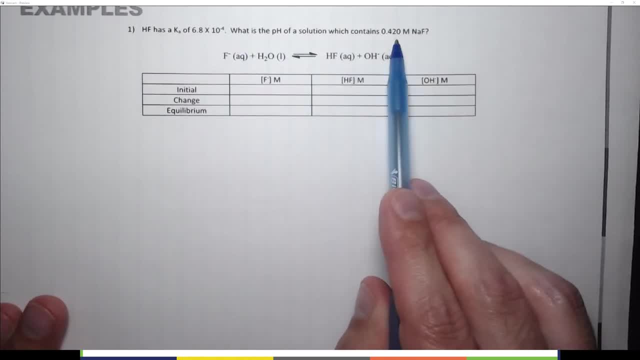 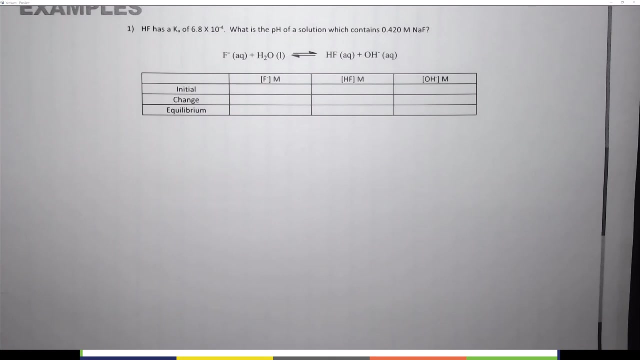 10 to the minus 4.. What is the pH of a solution which contains 0.420 molar NAF? It is not uncommon that you can only find KA values for some things, and if you can only find the KA value, sometimes you might need to calculate that. 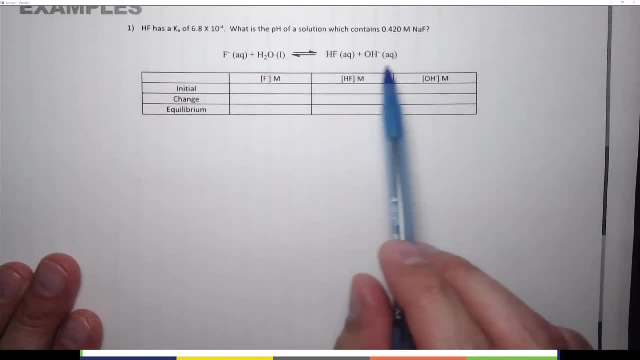 So we kind of have two ideas here. We have F minus plus H2O yields, HF plus or H minus. The NA isn't even written here. If you put the NAF and NAOH you'd get the same exact reaction. but it's not. 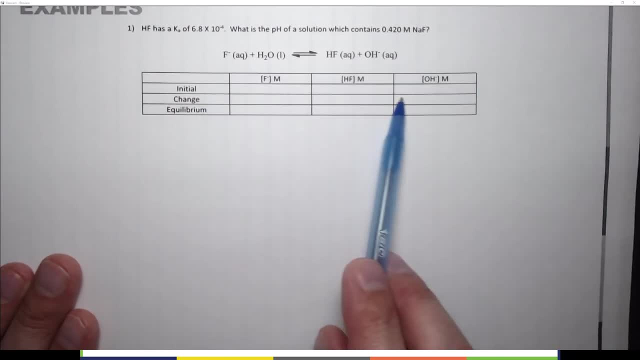 even written here, because it's just a spectator ion. And we have our ice table, which is set up as usual, But in this case we can't write a KA expression right, because this isn't a KA. F minus isn't acting as an ice table. So we're going to have to do a base problem. So we're going to have 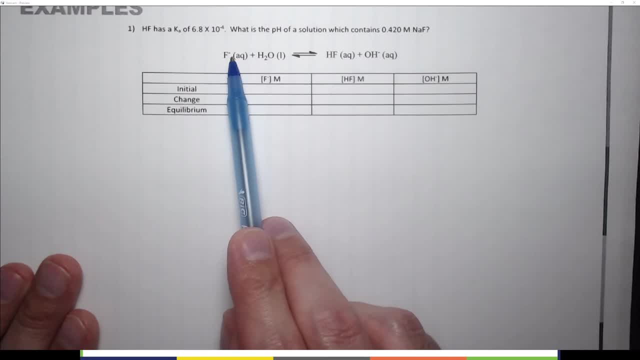 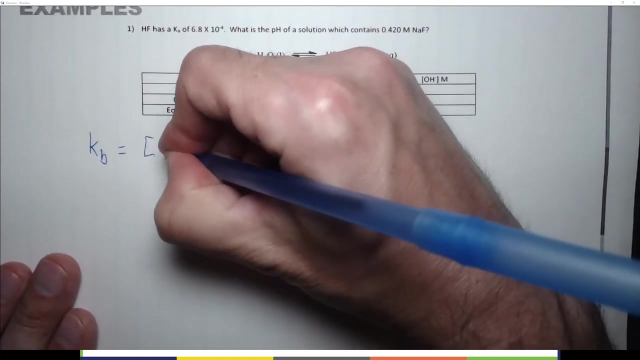 to write a KB expression because it's acting as an acid. It's acting as a base. So what we need to do is write a KB expression because it's forming OH minus in solution. It's not forming H3O plus in solution. So KB equals concentration of HF, the first product, concentration of OH minus. 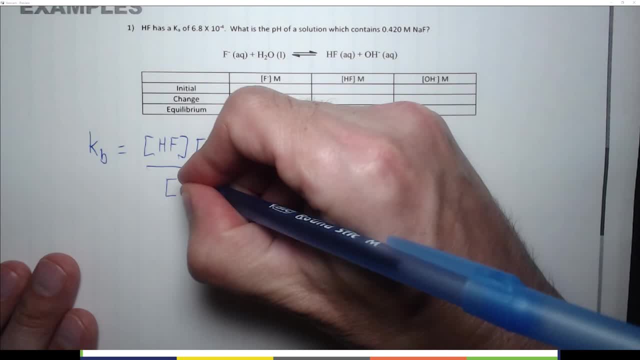 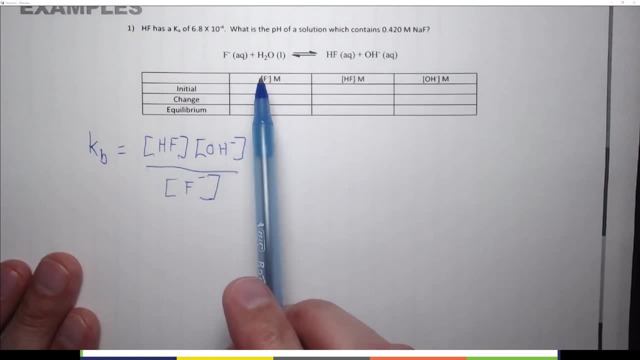 the second product over the concentration of F minus the reactant. But if you notice, here we ultimately want to find the pH of this solution, but we don't have pretty much anything we can do right. We don't have KB, We don't know HF, OH minus or F minus. So we need to start. 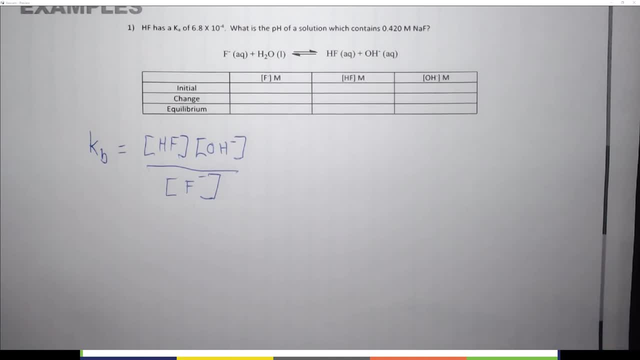 finding some of these things. It makes absolutely no difference which you start with. You could start with the ice table, or you could start by finding the KB. I'm going to start by finding the KB, but again, it doesn't matter, You can do it either way you want. Well, how am I going to find? 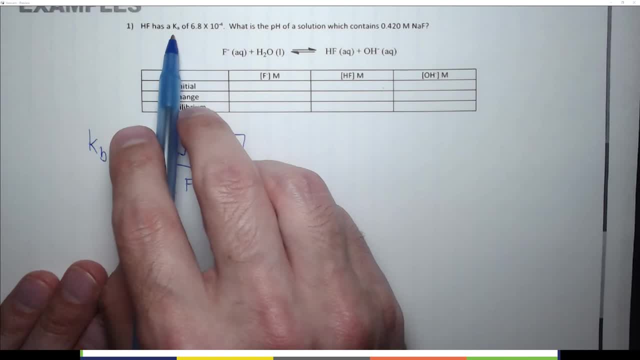 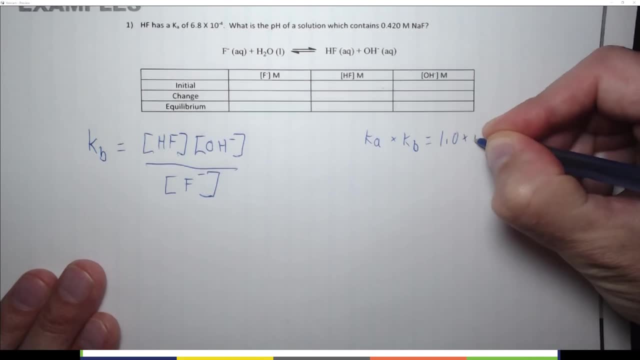 the KB. Not surprisingly, based on the previous question, I'm going to start by finding the KB. Next question: we're going to use the KA to do that. So, if you remember, KA times KB equals 1 times 10 to the minus 14.. Or said another way, KB equals 1 times 10 to the minus 14. 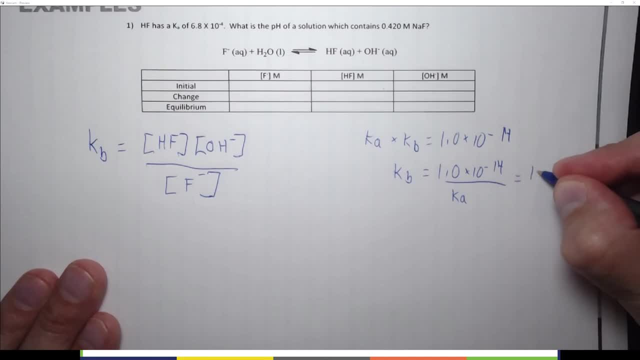 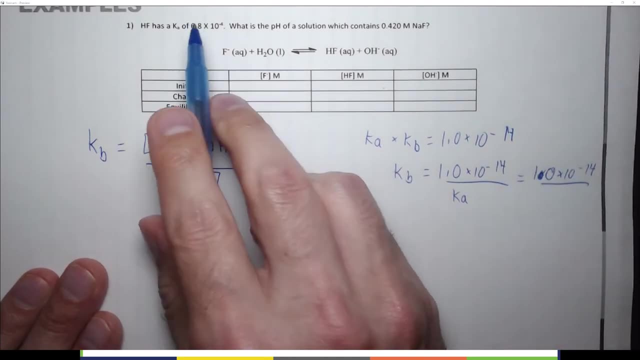 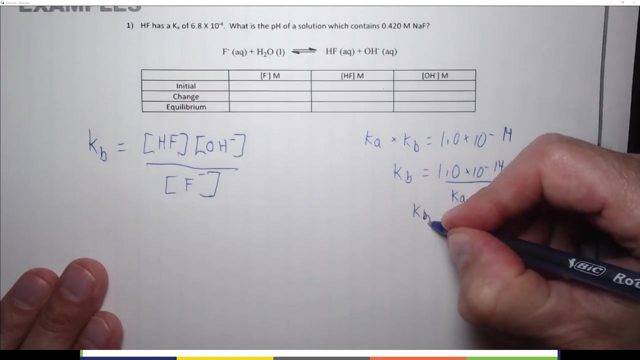 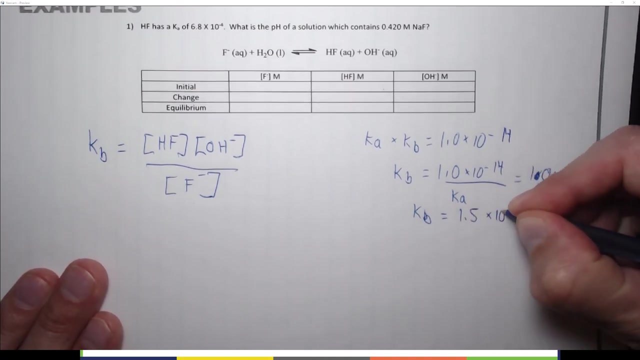 divided by the KA, which is 1 times 10 to the minus 14, divided by 6.8 times 10 to the minus 14.. So the KB here is equal to 1.5 times 10 to the minus 11.. All right, so I found the KB from the. 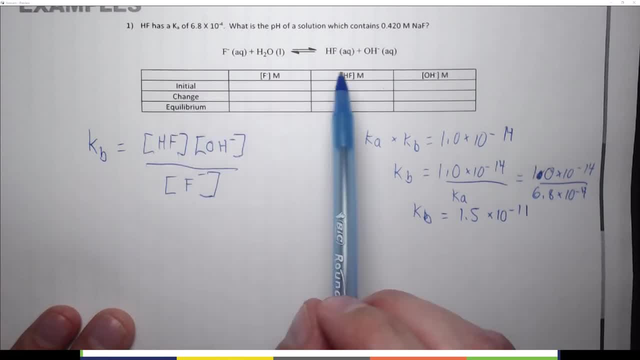 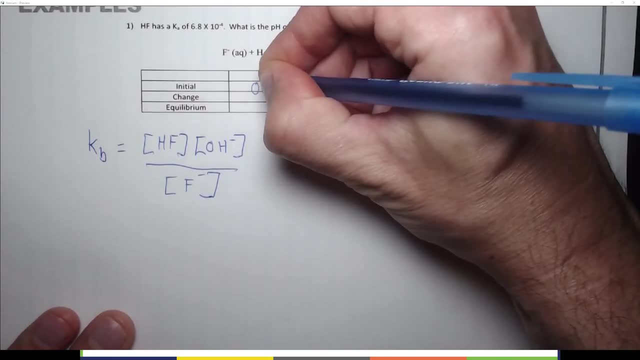 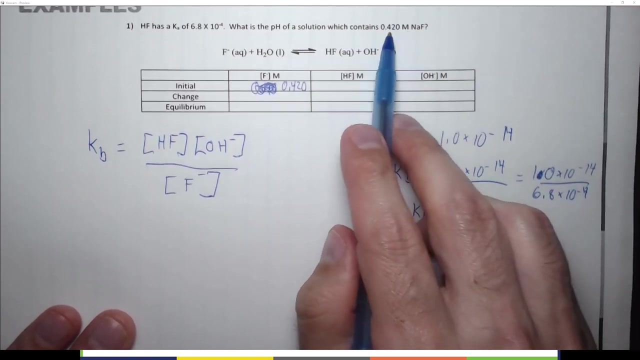 KA, just as in the previous question. Now I could set up my ice table. Well, the initial concentration of F minus is 0.42.. Try again: 0.42.. 0 molar, as given in the problem. Remember, the NA doesn't do anything. Okay, in this case, 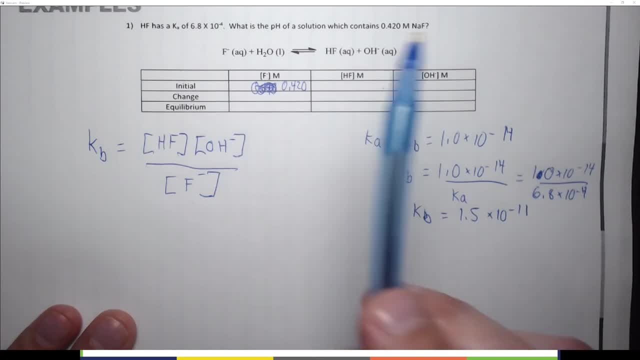 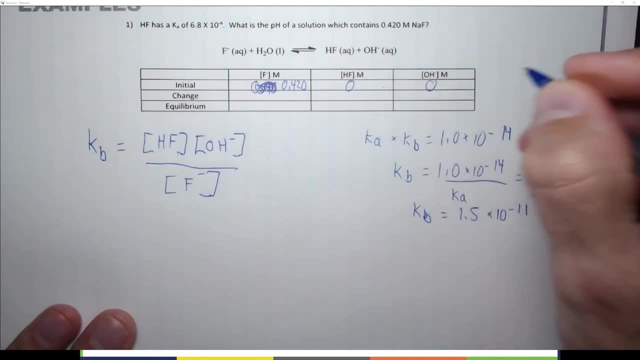 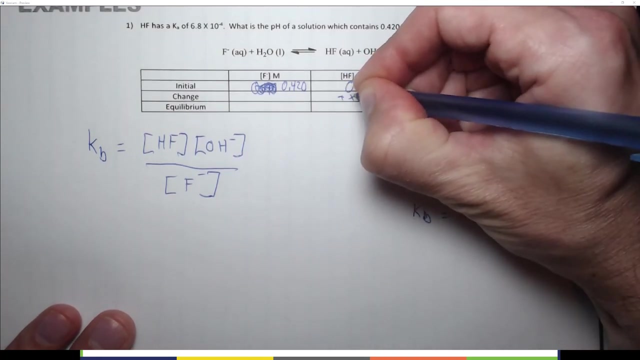 since it's one to one, every one of NAF you dissolve, you get one F minus HF. the initial concentration is 0 because we assume we start with only this And OH minus. we start with only this, So it's 0.. How much of HF and OH minus are we going to get? All right, we're getting the hang. 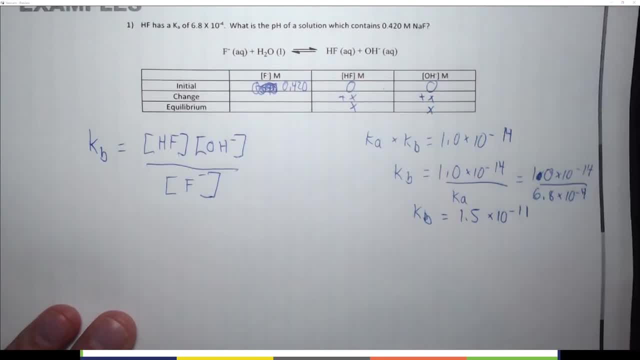 of this now. So it's just plus X. So we have X of this and x of this. Here we're going to subtract x and we're going to get 0.420 minus x Again, because the stoichiometry is all one-to-one. they're all just x's, which, again, we're going. 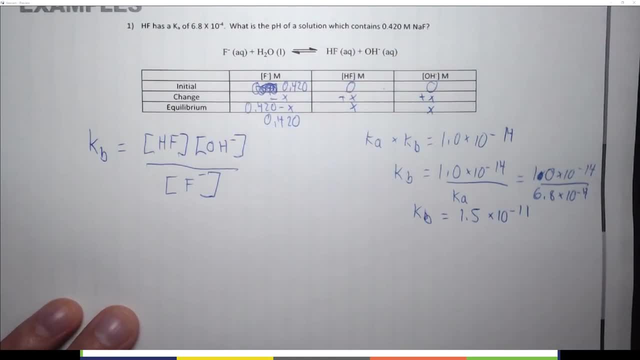 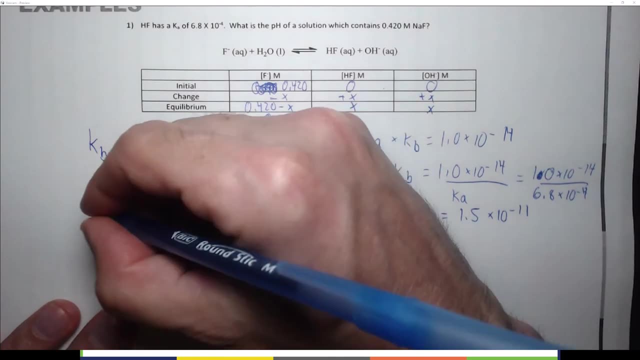 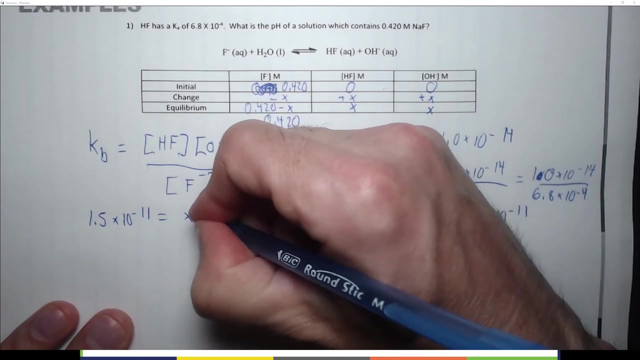 to assume is just 4.420, and that this is less than 5%. Okay, so now I can set this up because I have my variables. I have KB 1.5 times 10 to the minus 11,. okay, equals x times x divided by. 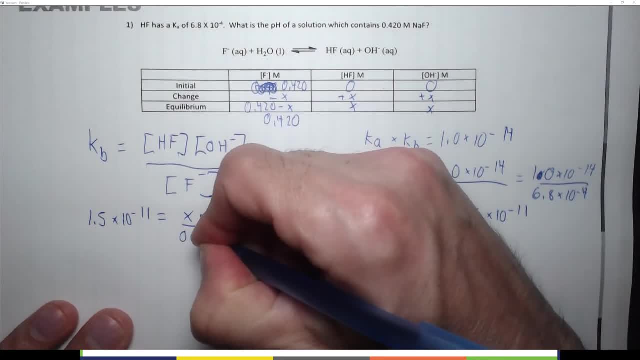 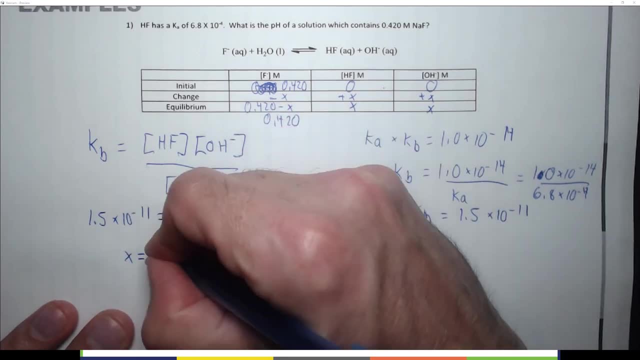 f minus, which is 0.420.. When you do all that math, you find that x is equal to 7.8 times 10, to the minus 6.. All right, I didn't show you how I got there, because I've showed you. 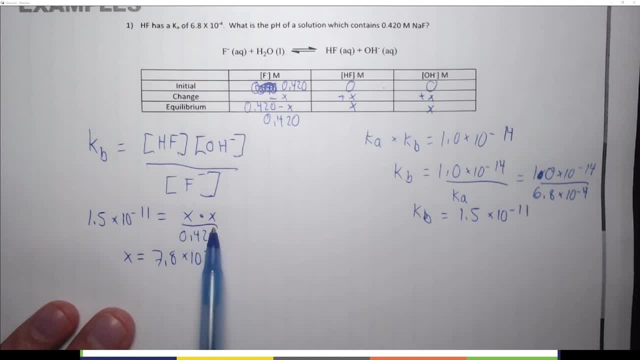 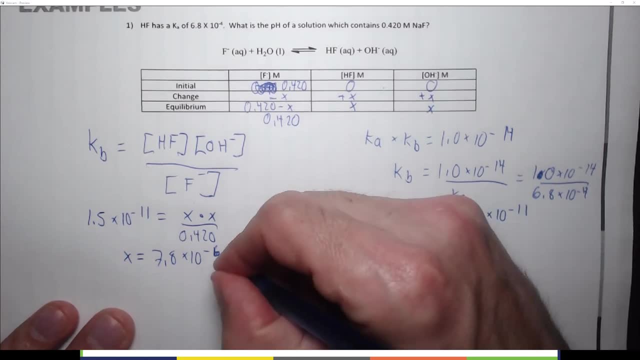 how to do it. I'm not going to show you how to do it. I'm going to show you how to do it. get there um three or four times before. so i just went directly across, multiplied, i took the square root and i get 7.8 times 10 to the minus 6. well, what is this? the concentration of this is the. 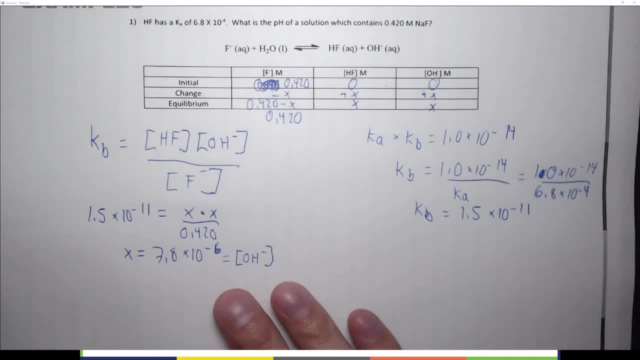 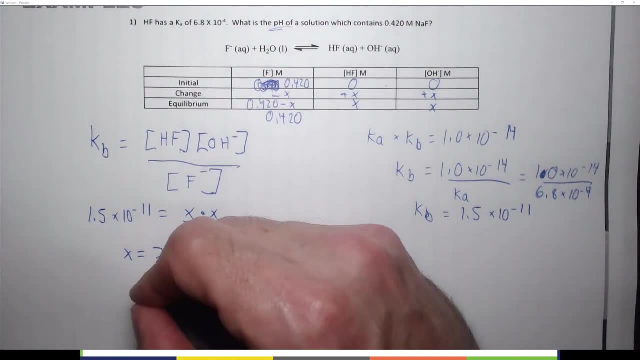 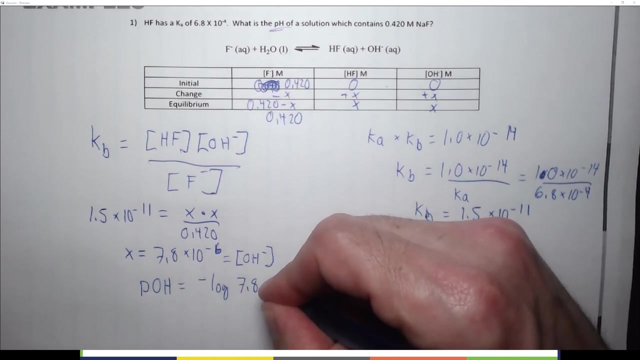 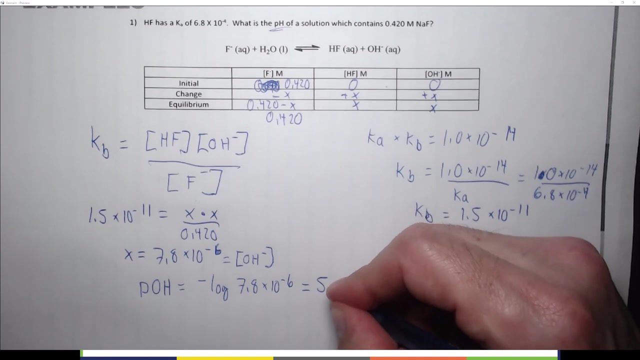 concentration of oh, minus. well, what can i do with that number? well, remember that my goal is to find the ph. so what am i going to do with that? first, i'm going to find the poh, and the poh equals the negative log of 7.8 times 10 to the minus 6, which is equal to um 5.60. then to find the ph.